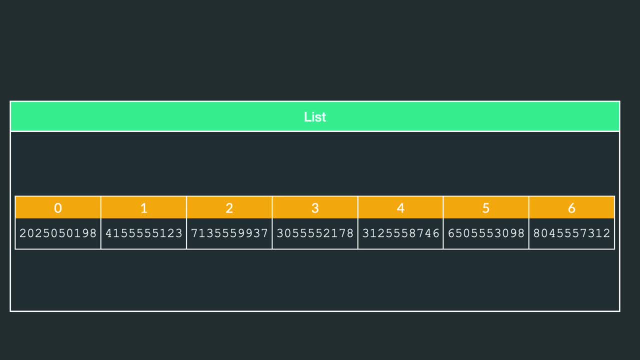 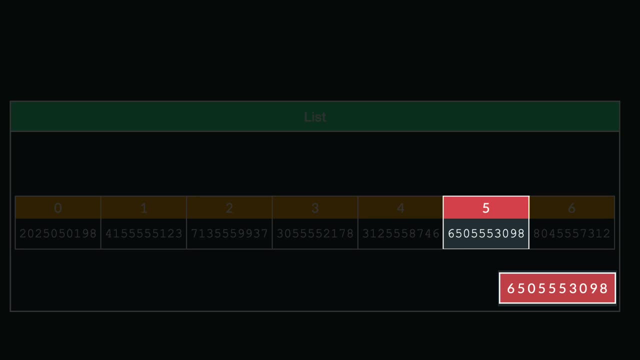 The straightforward approach would be to store the phone numbers in a list and then compare each element against a target value, one by one, until you find your match. This is called linear search and it works well for small datasets. but with a large database like a million records, searching through it one by one would be very slow and 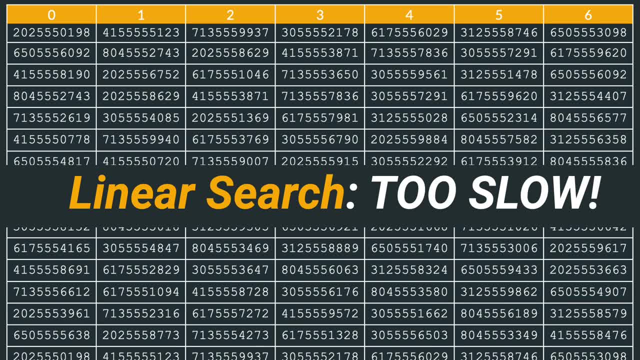 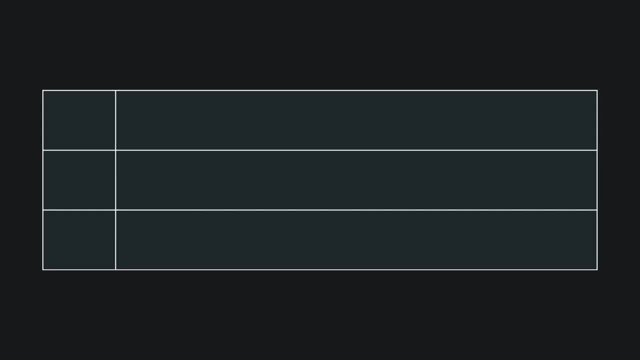 very inefficient, So Hans suggested a more efficient approach. Instead of storing phone numbers in a plain old list, he proposed dividing them into buckets, And to determine the bucket that a phone number would belong to, Hans would apply a mathematical operation. This operation groups the digits into pairs, adds them up and keeps only the last digit. 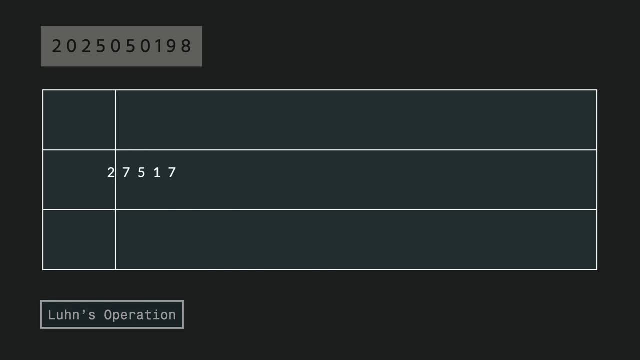 if a number has more than one. The original phone number is then placed into a bucket that matches the final result, Although this phone number is different. applying Hans' operation would be much more efficient and it would be much easier to find the number that matches the final result. 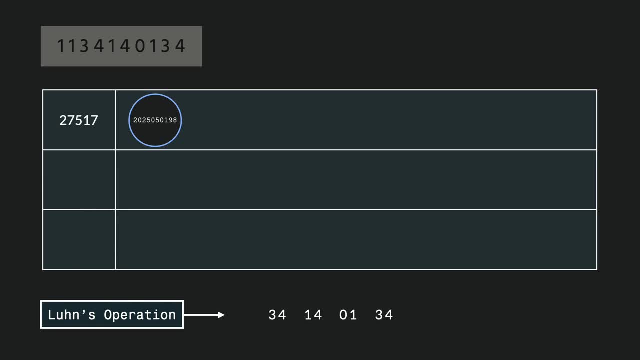 This operation would be much more efficient and it would be much easier to find the number that matches the final result. So Hans suggested a more efficient operation of pairing the digits, taking the sum and keeping only the last digit. if there happens to be more than one will still place it. 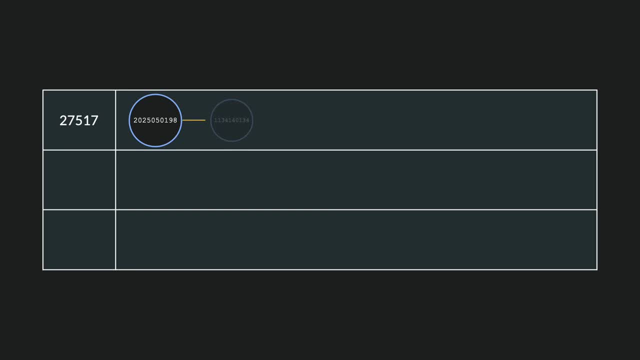 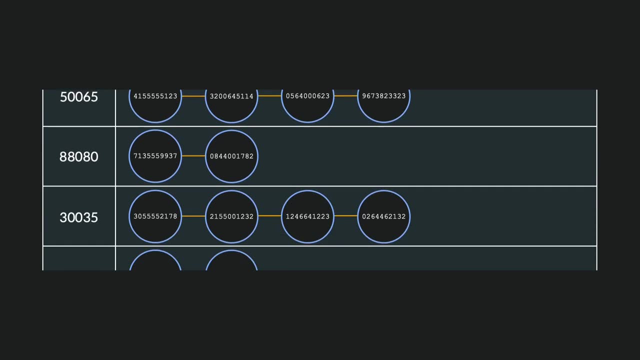 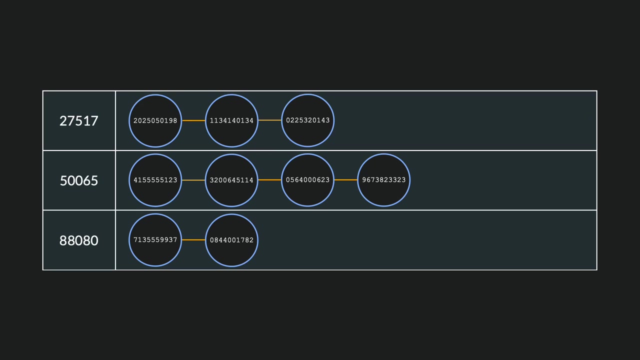 inside the same bucket. I will apply this process to 15 phone numbers, resulting in a total of 5 buckets for all 15 numbers, And I hope you can see how dividing the database into these buckets significantly reduces the searching space, Because if there is a target phone number to find, then I can apply the same mathematical. 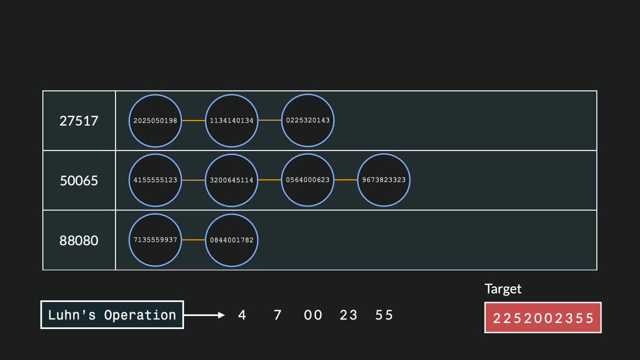 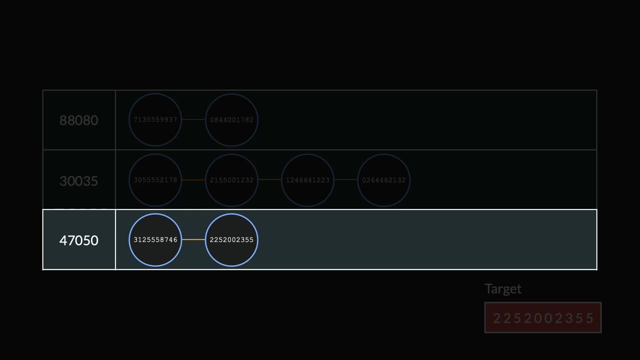 operation to determine the bucket that contains it. And now, instead of looking through 15 phone numbers, I only have 5 buckets to look through. Once I find the bucket that the phone number is in, I only have to compare the phone numbers. 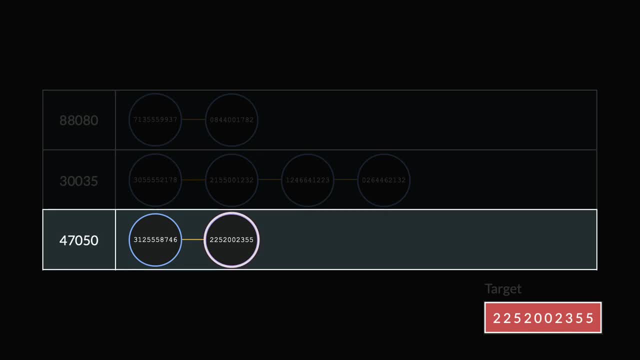 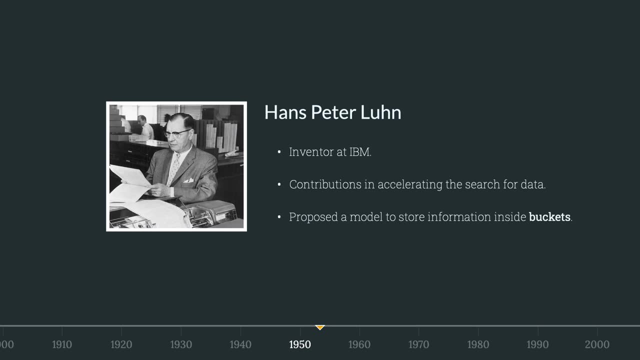 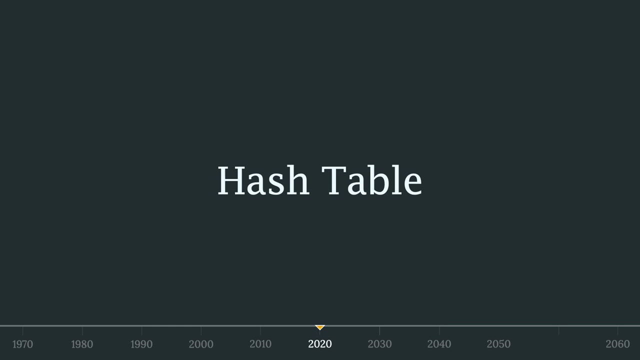 within the bucket to my target value and return the phone number that matches it. This method of storing data in a table of buckets is a precursor to the hash tables that we commonly use today. So as we look at the inner workings of a modern day hash table, you're going to notice many 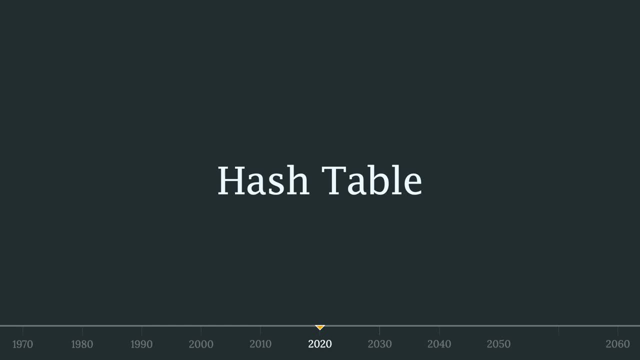 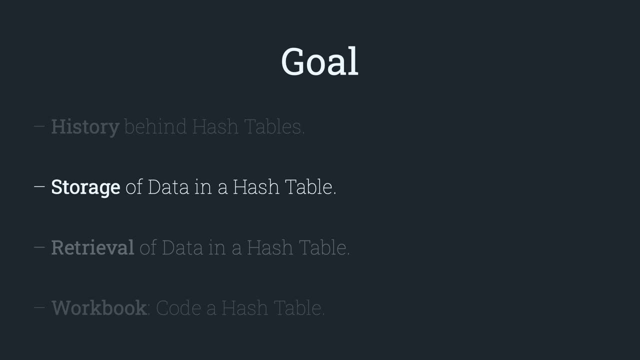 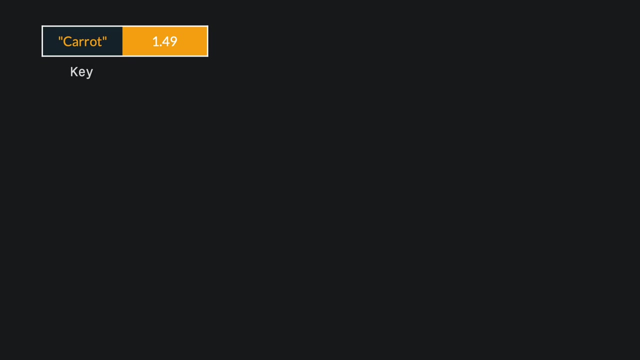 similarities to Hans's model. First, we're going to go through the process of storing data in a hash table. You can store entries in a hash table. An entry is a key-value pair. The key is used to locate a specific piece of data, while the value represents the actual. 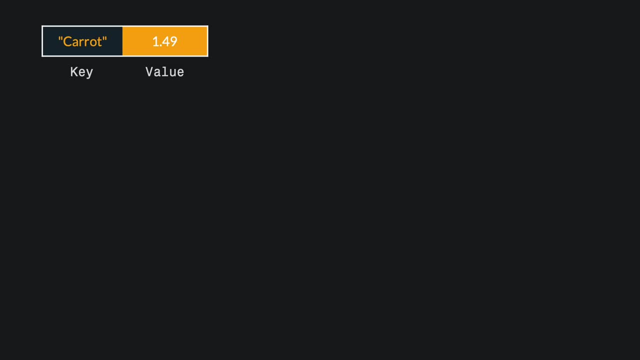 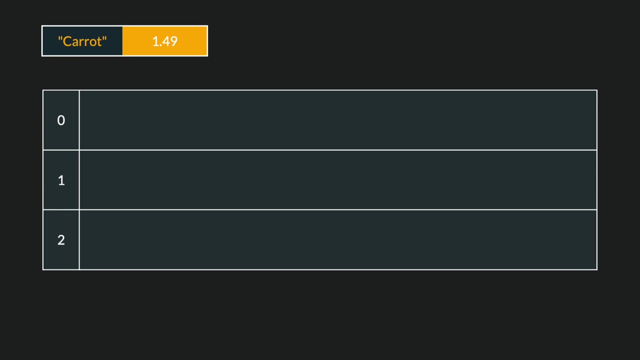 data of interest. Internally, the hash table is supported by an array of buckets. At first, the array doesn't have the capacity to store anything. However, as we insert the first entry into the hash table, the array must be resized to accommodate the new data. 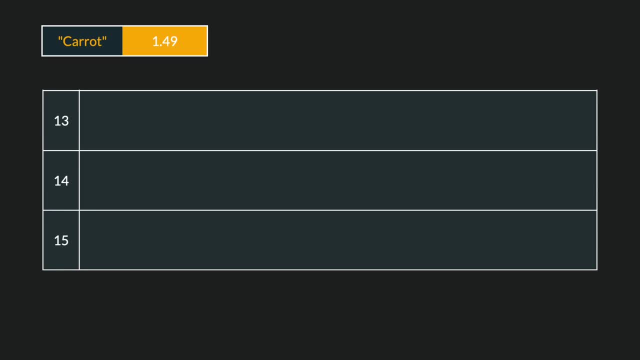 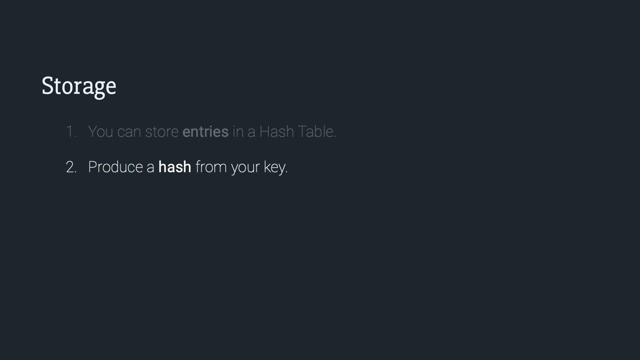 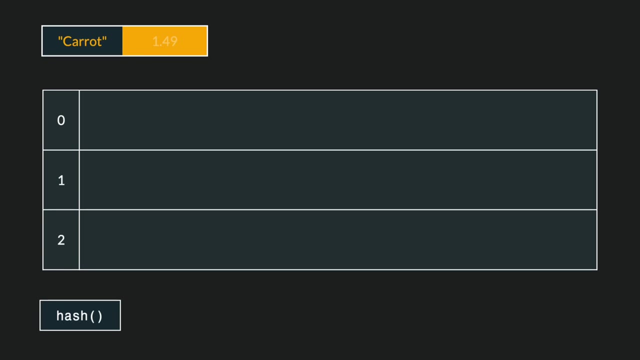 For this particular hash table, an initial capacity of 16 has been assigned, where the capacity represents the number of available buckets. Step 2 is to produce a hash from your key. A hash function is a mathematical operation that takes a key as input and generates a. 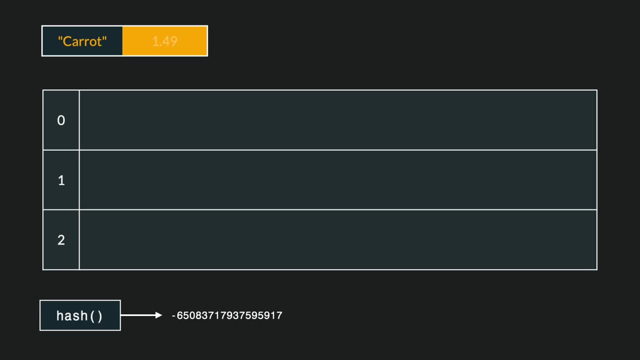 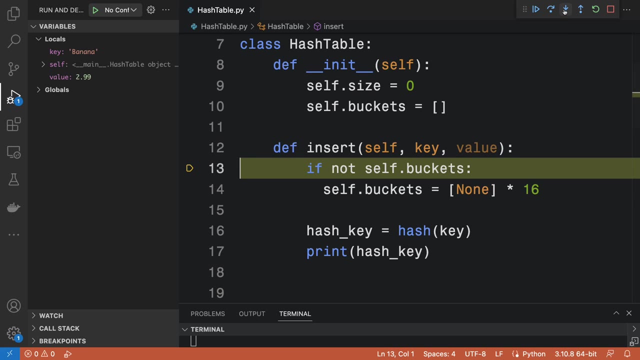 unique value known as a hash. The hash value will be unique for different inputs. We insert our first entry, a banana for $2.99.. Because this is the very first entry, the hash table is going to start by resizing to 16 buckets. 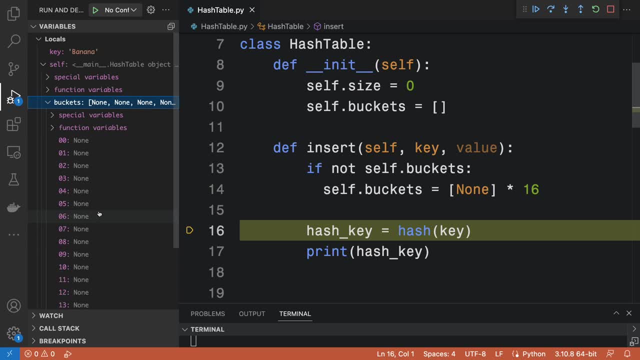 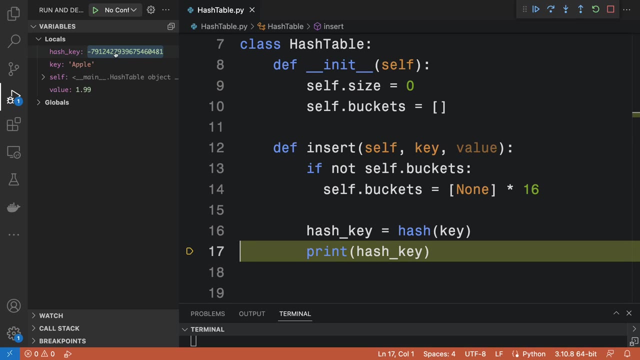 We can confirm that, Then the hash function is going to process the key and produce a hash. We can repeat this process for two more entries and you'll notice that the hash value is going to be unique for different inputs. And here we've got the hash value for lime. 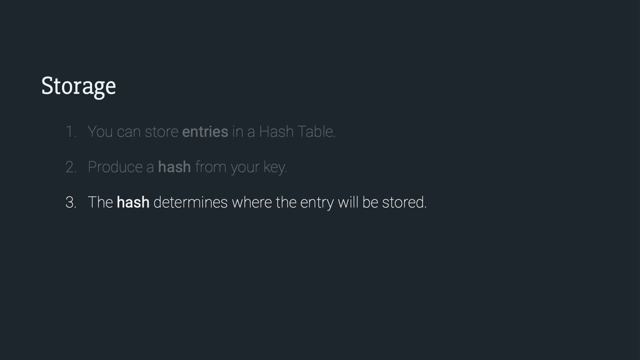 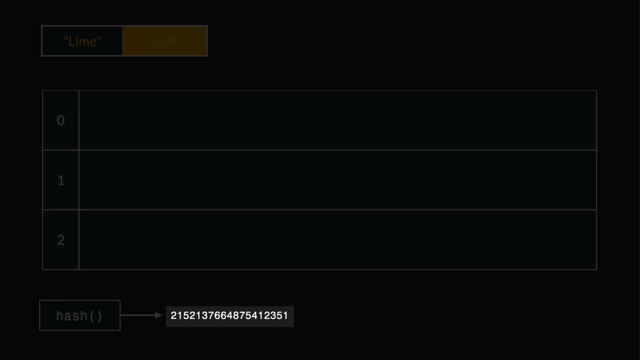 The hash of a key determines where the entry will be stored. The hash value that corresponds to the key lime is, in this case, 2 quintillion. And somehow, from this hash value, from this astronomical number, we need to extract an. 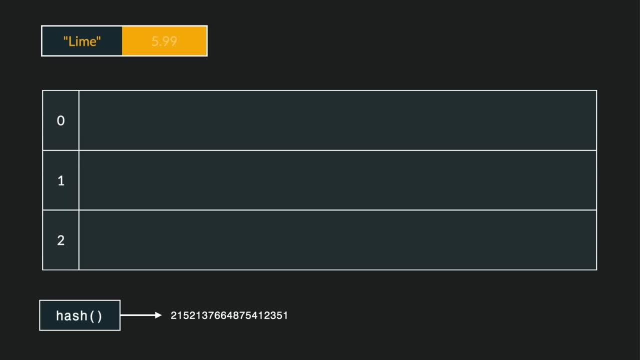 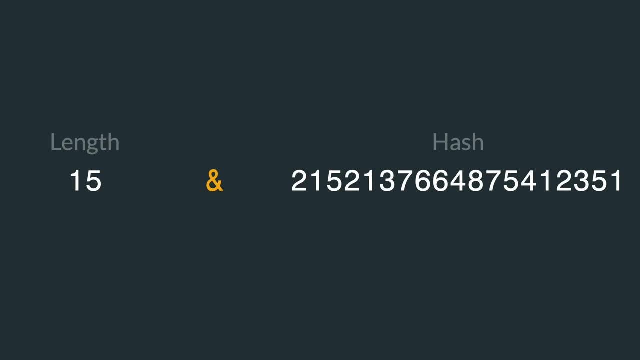 index that ranges from 0 to 15.. This can be achieved by performing a bitwise AND operation between the length of the array and the hash value itself. Performing a bitwise AND operation involves representing both numbers in binary form, 0s and 1s. 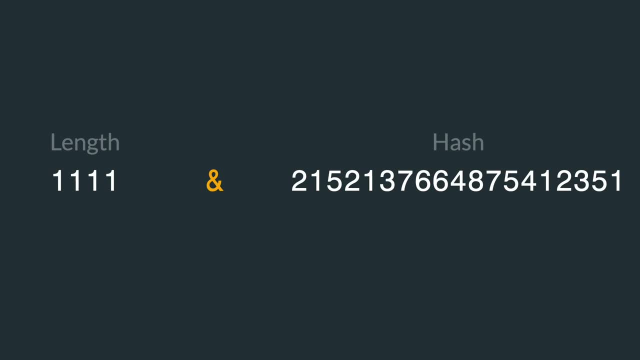 15 in binary 4: 1s, The hash value 2, quintillion- in this case in binary, is this monstrosity. And since the first binary number only has 4 bits, we can ignore all the bits in the. 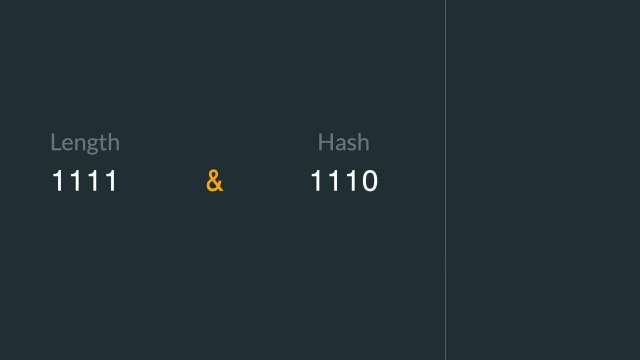 second binary number that come after the first, 4.. And the way a bitwise AND operation works is that if both numbers are 1, the result will be 1.. If either of the numbers is not 1, the resulting value is 0.. 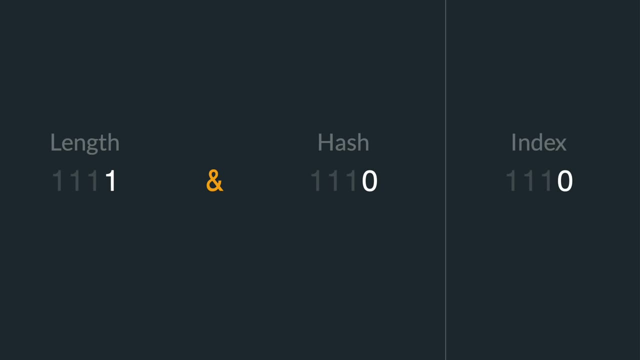 If either of the numbers is not 1, the resulting value is 0.. If either of the numbers is not 1, the resulting value is 0. And, remarkably, the operation produces a valid index. The reason for this is that the bitwise AND of any two numbers will always produce a number. 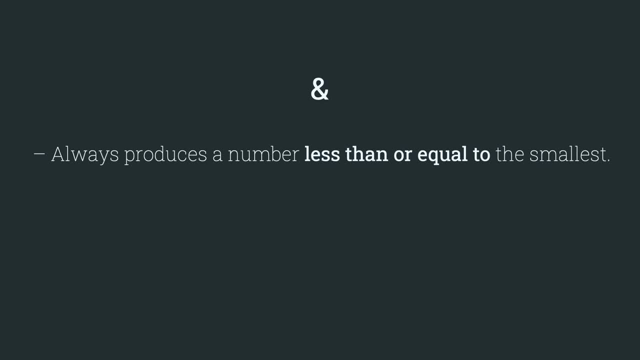 less than or equal to the smaller 1.. Therefore, by performing a bitwise AND operation between the two numbers, the result will be 0.. 1., 1., 2., 3., 4., 5., 4.. 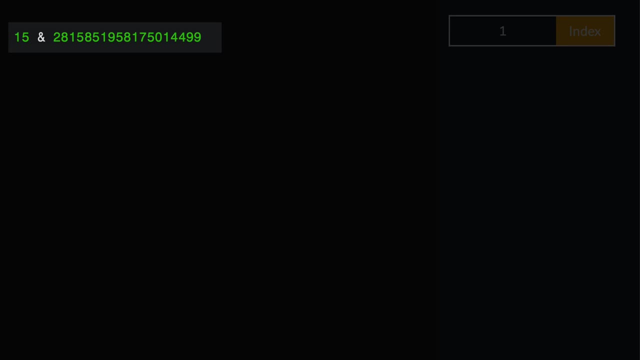 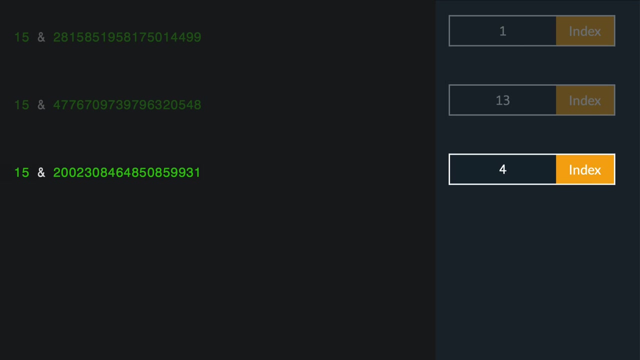 5., 6., 7., 5., 6., 7., 8., 7. a bitwise AND operation between the length of the array and the hash. the resulting value will always be less than or equal to the length of the array. This guarantees that the index calculated. 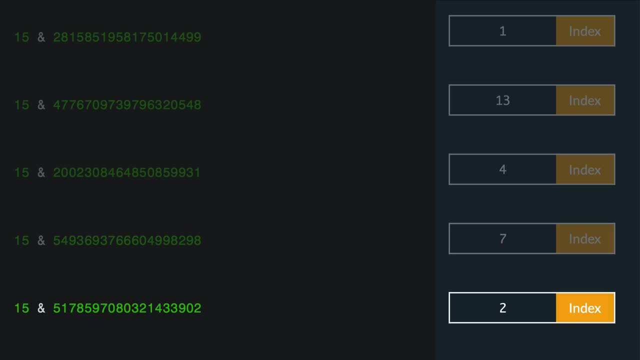 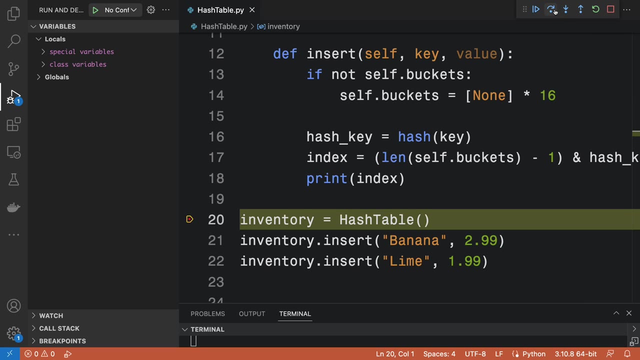 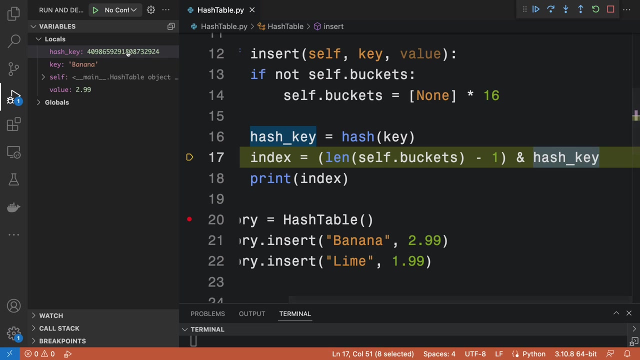 from the hash will be in a valid range of 0 to 15.. We can start by inserting the banana. We will step through the code from before And here I've got the hash value for banana. If we perform a bitwise AND operation between the length of the array against the really large, 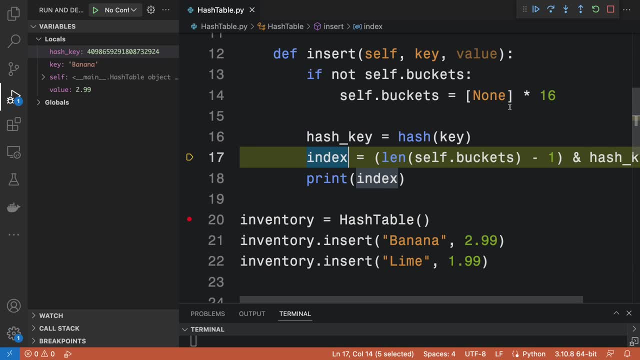 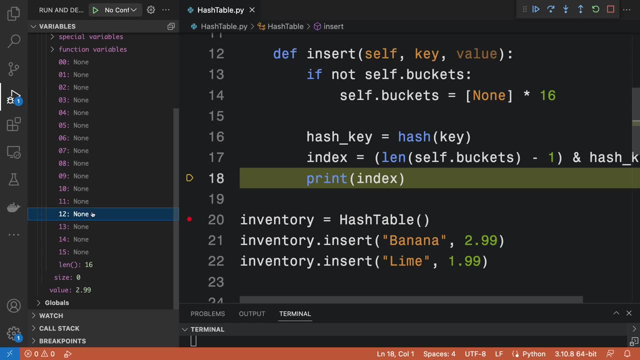 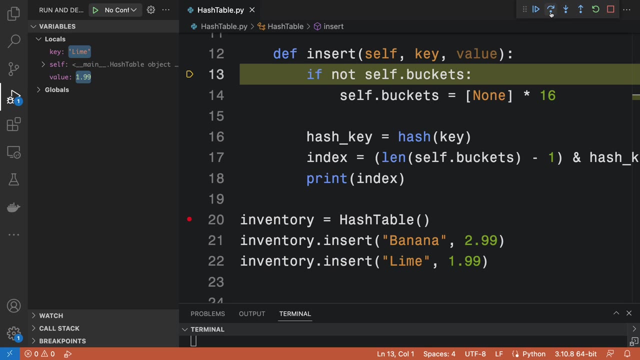 hash value that's going to guarantee a valid index inside the bounds of the array. so banana would have been placed inside index number 12 of our buckets array. We can repeat this one more time for lime, Once again stepping through all the code from before. 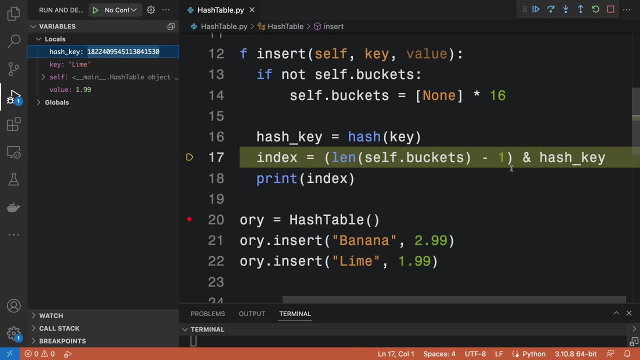 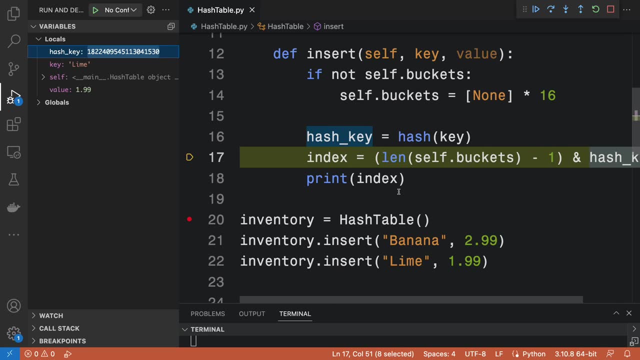 Here we've got the hash value for lime. Performing a bitwise AND operation between the length of the array and the hash, the resulting value will always be less than or equal to the length of the array and the hash. the resulting value is going to guarantee a valid index inside the bounds of the buckets array. In this case, 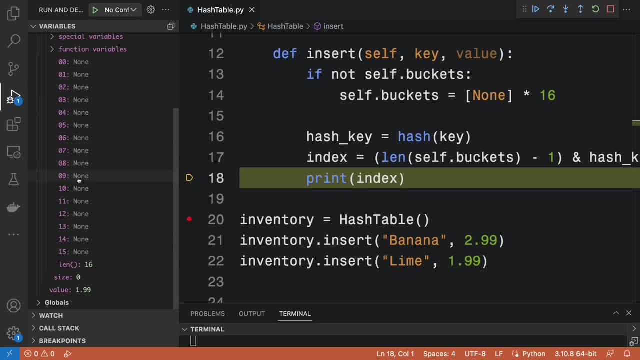 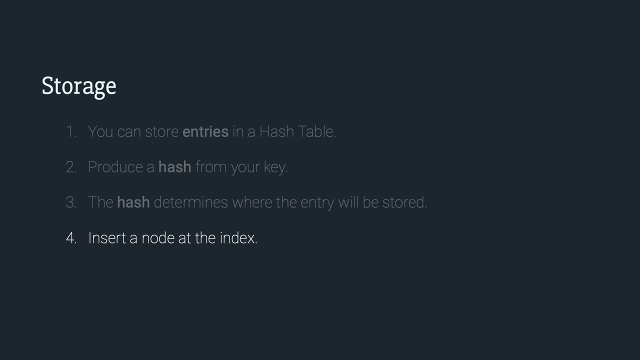 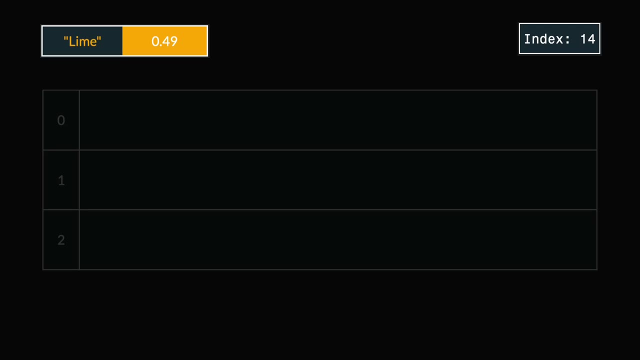 the lime entry would have been placed inside of bucket number 10.. Step 4 is to insert a node at the index that you calculated. So, after determining the appropriate index for the entry, you can store the key value pair in the form of a node. 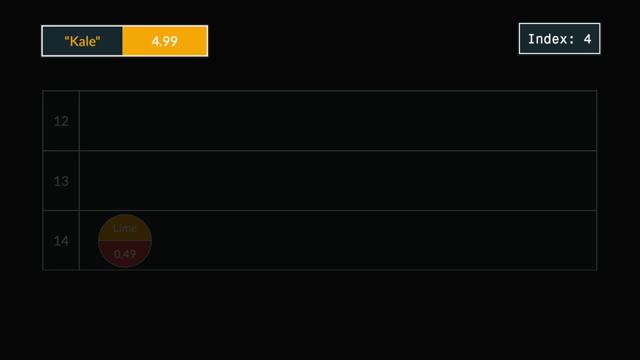 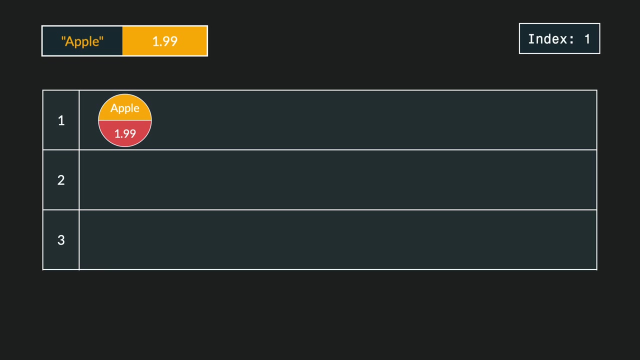 In this case, the hash of the kale key determined that it should be in index 4.. And here the hash of the apple key determined that it should go in index 1.. The first entry we're going to insert is papaya for 299.. 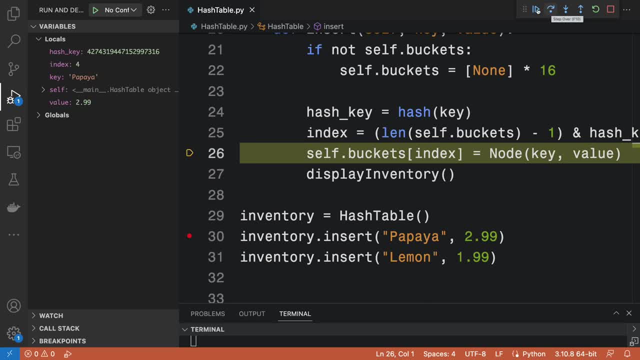 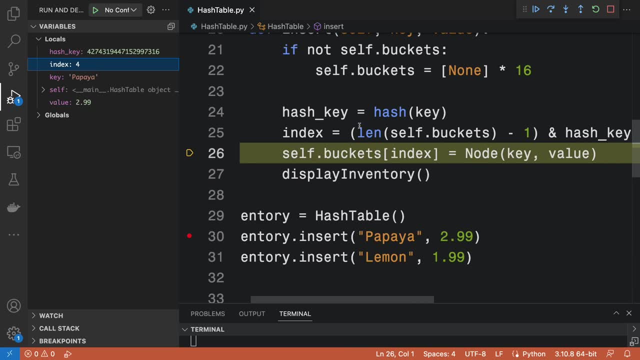 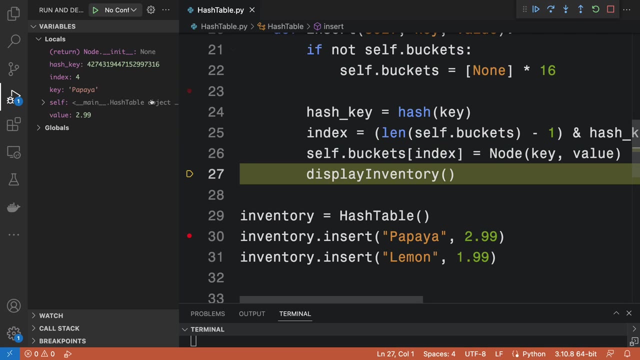 Skipping through all of these lines, the hash of the papaya key is going to determine that it should be placed inside of bucket number 4.. So here what we do is we store the key value pair in the form of a node and then insert the node inside of the hash table at the appropriate 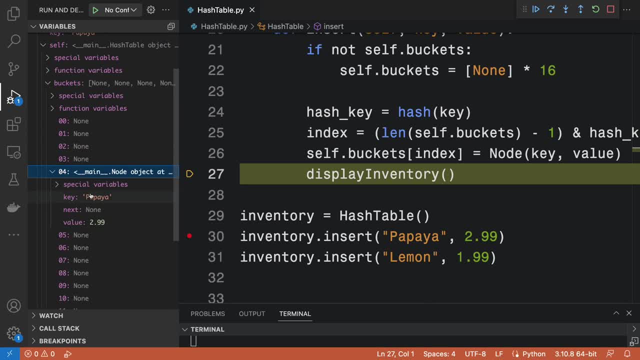 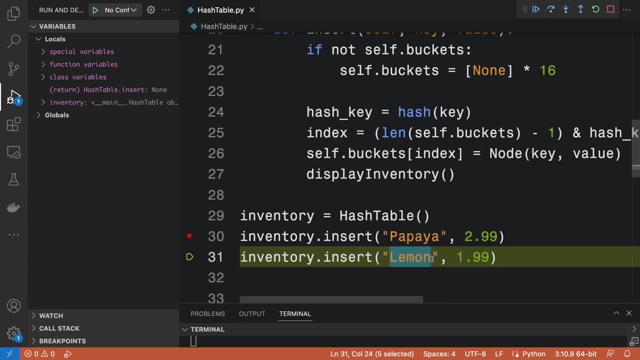 index. Here we can see papaya for 299 is inside of bucket number 4. Beautiful. Let's look at another example. Here we insert lemon for 1.5. And here we can see lemon for 1.99.. Skipping through all of these lines because the hash of 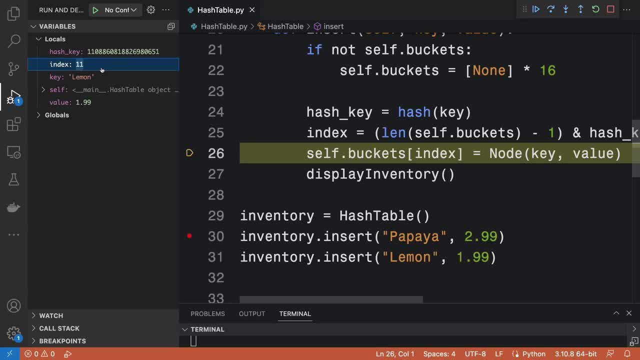 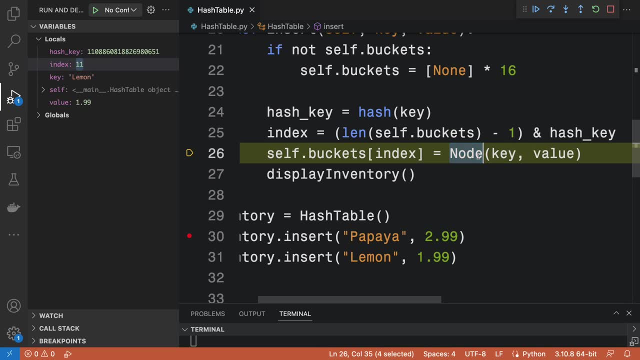 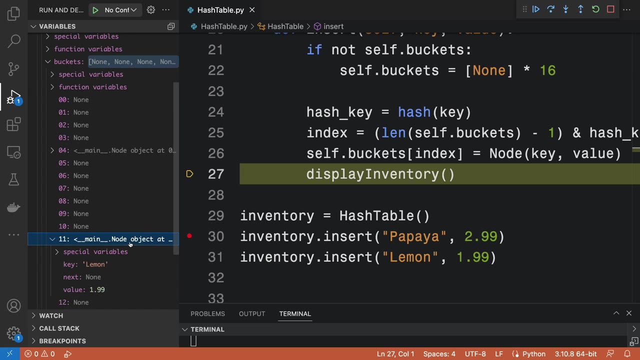 the lemon key is going to determine that it should be placed inside of index number 11.. So we store the key value pair lemon for 1.99 in the form of a node and then we insert that node inside of our buckets array And here we can see our entry is inside of bucket number 11.. 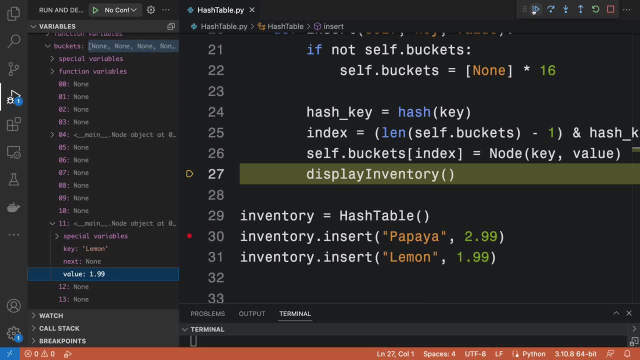 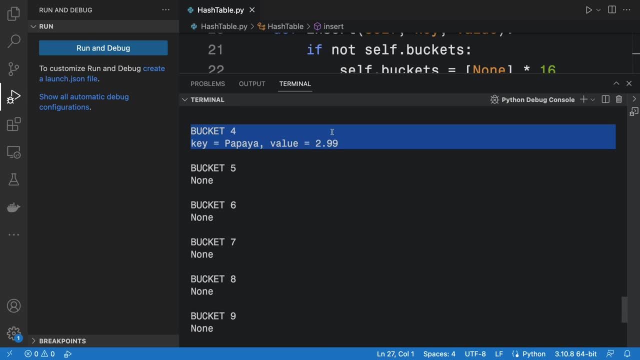 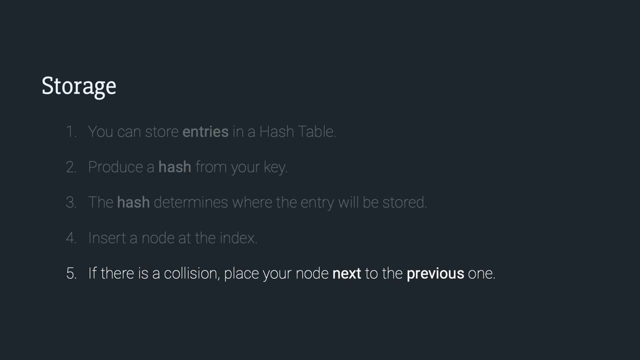 And after executing this line, we can display the inventory inside of our terminal And visualize our buckets Beautiful. Finally, in the event of a collision, place your node next to the previous one. A collision happens when the hash of a key produces an index that already contains a node. 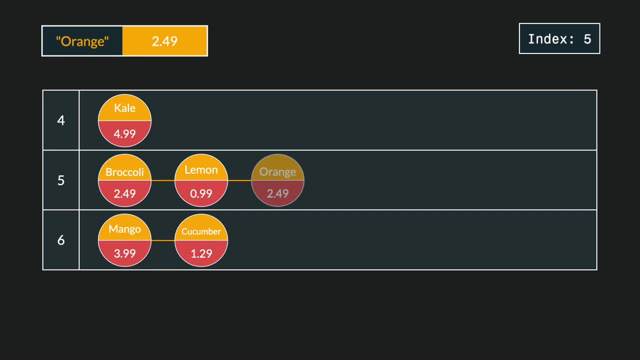 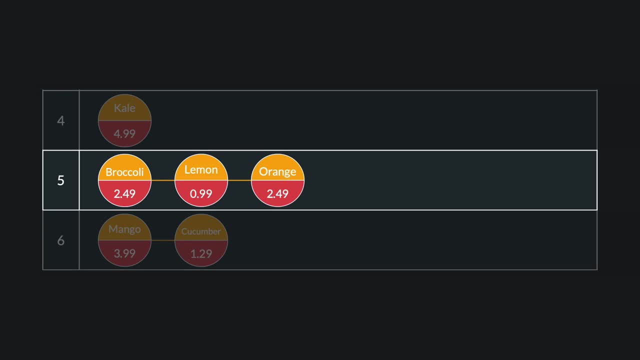 At this point you can insert the new node. It follows that every element in a hash table points to a list of nodes, also known as a linked list. We can start by inserting the banana entry, skipping once again the lines from before. 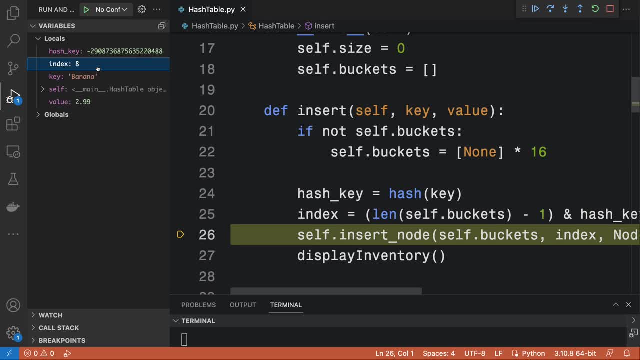 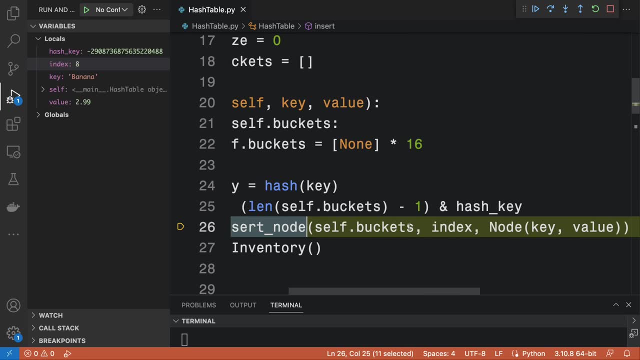 The hash of the banana key is going to determine that it should be placed inside of index number 8. And what we're going to do is rely on a special method called insertNode to insert our node at the appropriate index inside of our buckets array. 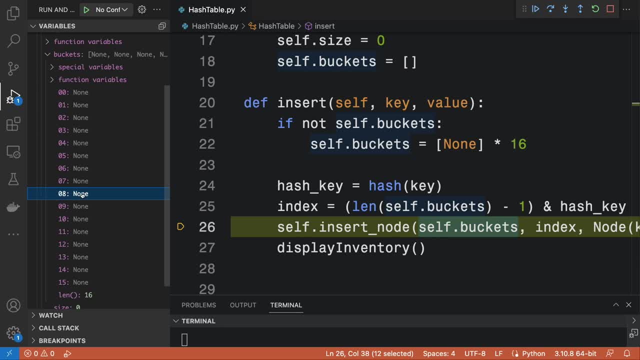 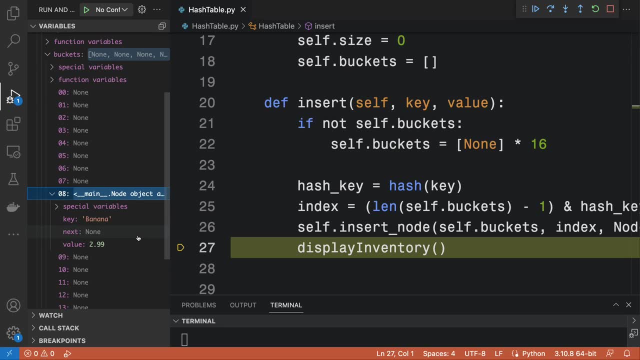 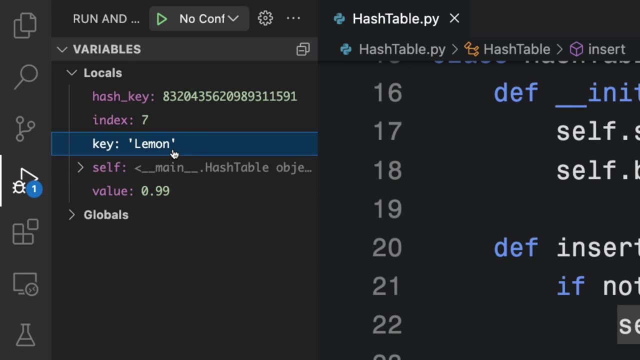 Because the bucket at the given index of 8 is empty. it's simply going to place the node at that index. Very simple, Let's fast forward a bit Now. I'm in the process of inserting an entry with a key of lemon and a value of 99 cents. 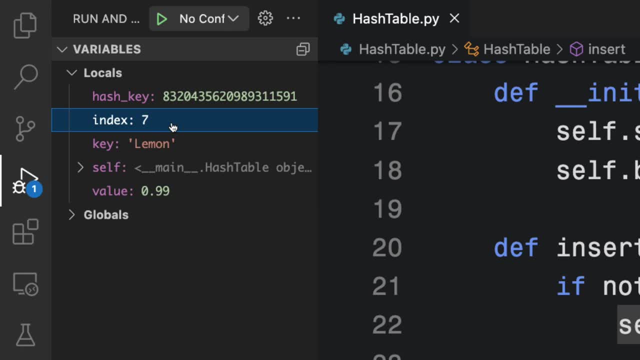 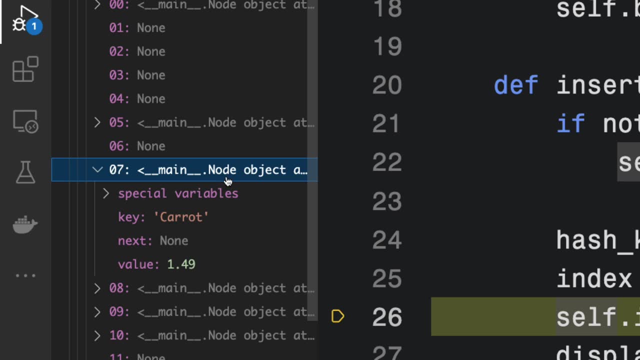 The hash of the key determined that it should be placed inside of bucket number 7.. But bucket number 7 already contains a carrot node. Because this bucket is not empty. what insertNode is going to do is add our new node next to the previous node. 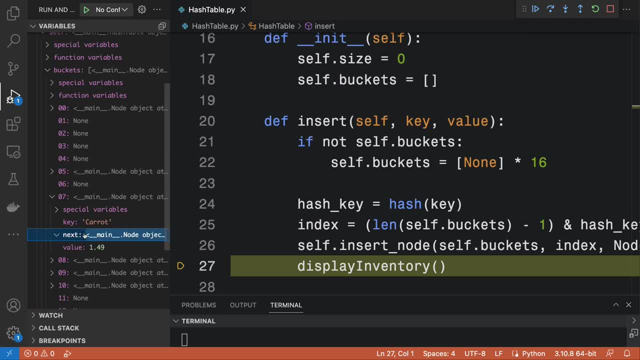 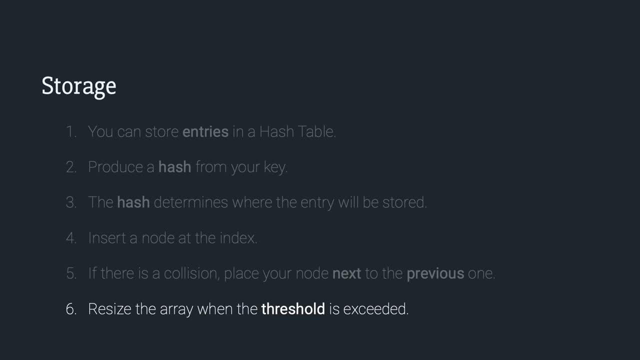 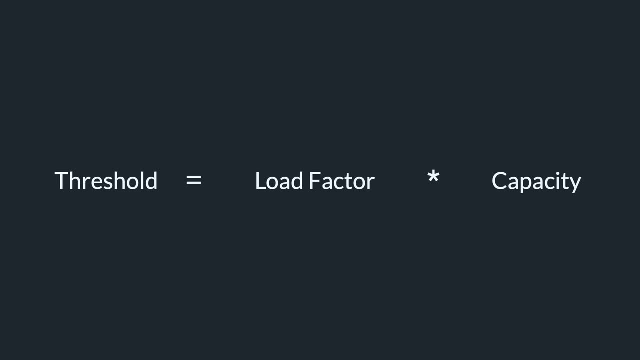 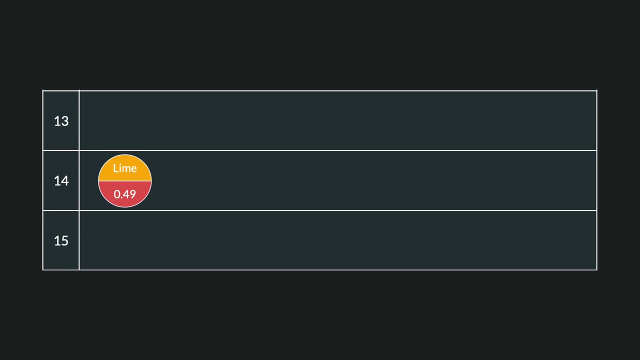 So bucket number 7 first contains carrot and next to it we see the lemon node. Step 6 is to resize the array when we exceed a particular threshold. The threshold is equal to a load factor multiplied by the capacity of the array. There are 16 buckets, so the current capacity of the array is 16.. 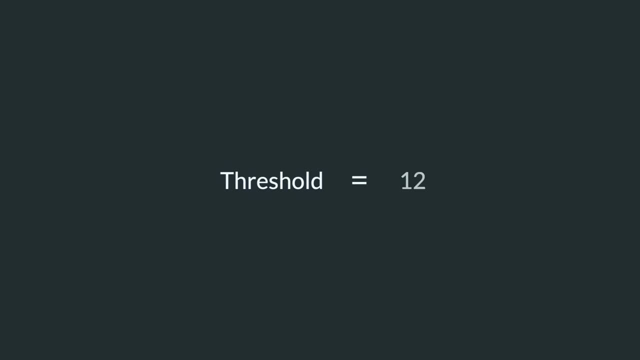 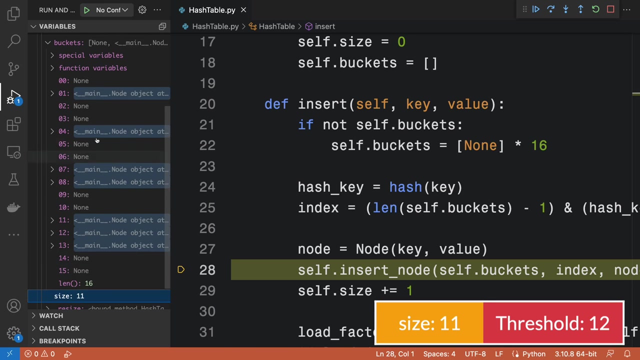 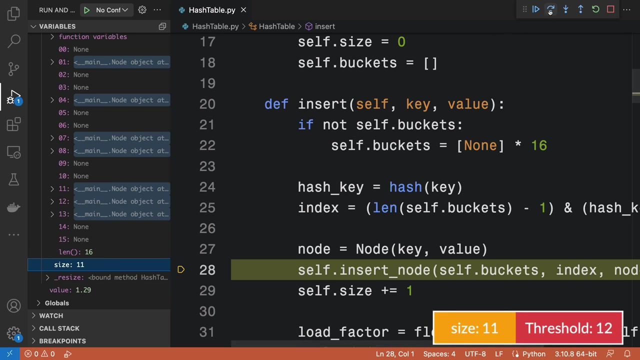 With a typical load factor of 0.75,, our threshold before the next resize is 12.. At this point, I have inserted 11 nodes inside of my buckets array, the size is 11, and so, after adding one more node, the size is going to be 12.. 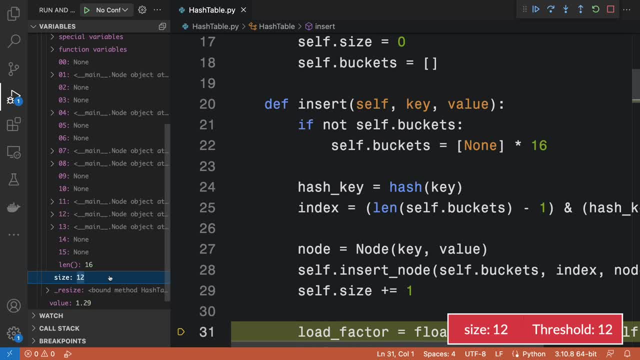 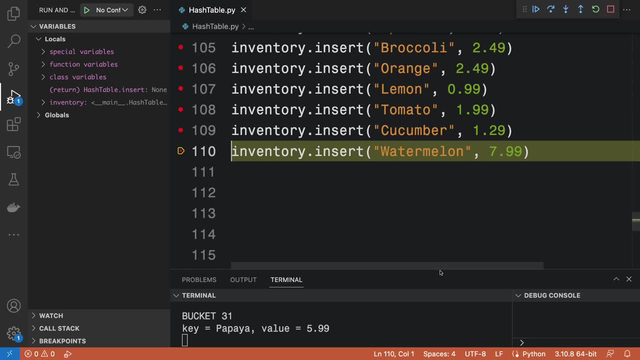 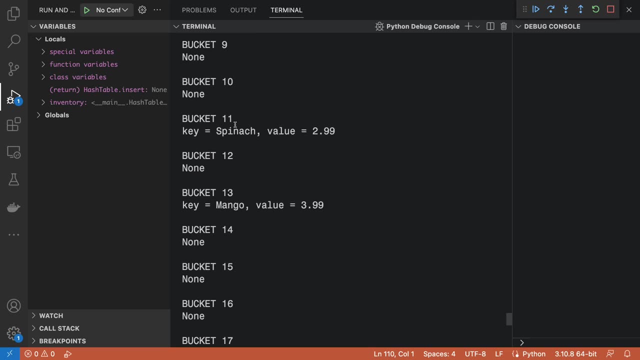 And now that the size has reached the threshold, we're going to tell our hash table to resize. We can now display our new hash table And you can see all entries from the previous hash table were reprocessed and re-indexed into the new and much bigger one. 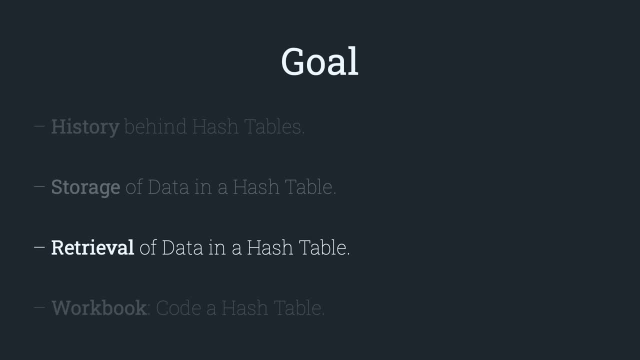 Great. we can now proceed with part 3 of our video, where we will see how we can add a new hash table. In this video, we will discuss how to retrieve data from a hash table. In order to retrieve data, you need to know the key that maps to the value that you're interested in. 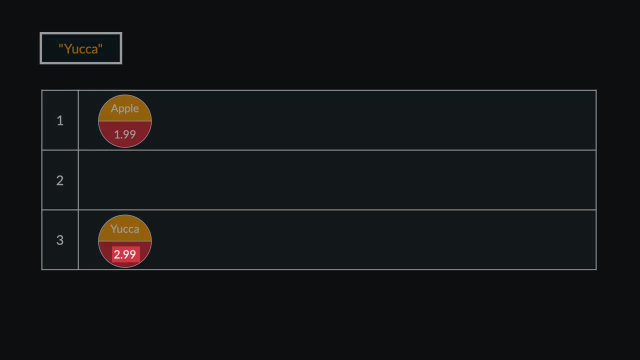 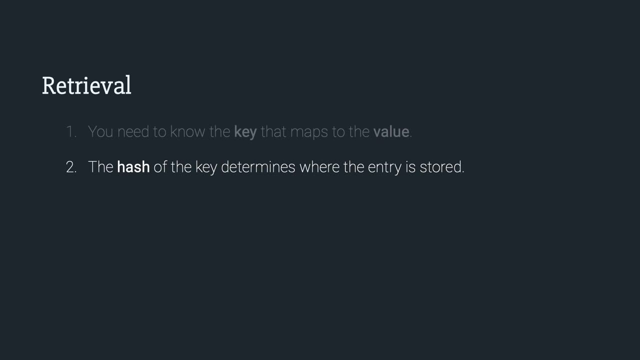 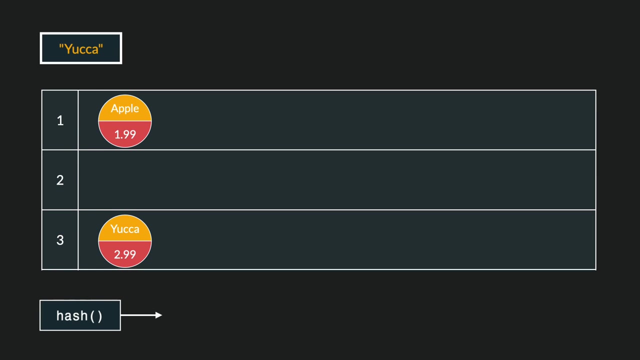 For instance, by passing in the key for yuca. the goal is to retrieve its price value And you'll remember that the hash of a key determines where the entry is stored. The key gets processed by a hash table. The key gets processed by a hash function to produce a unique value known as a hash. 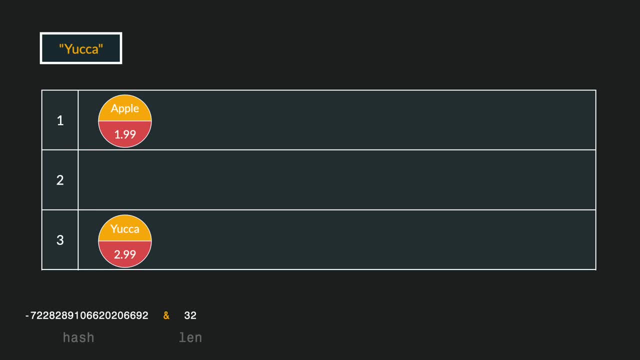 The bitwise AND operation between the hash and the length of the array determine the index where the entry is stored. We found the bucket that yuca is in The first node inside the index matches the key yuca, so we can return its value. 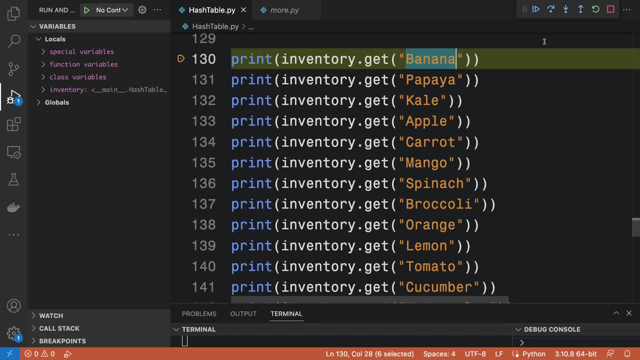 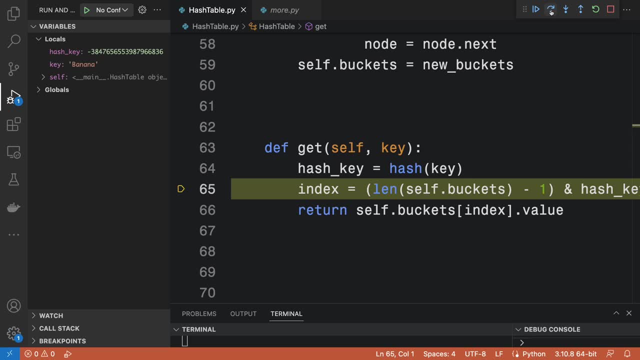 First we want to get the value that corresponds to the key banana. so we step inside of the method. The key gets processed by a hash function to produce the unique hash that corresponds to the key banana. The bitwise operation between the hash and the length of the array is going. 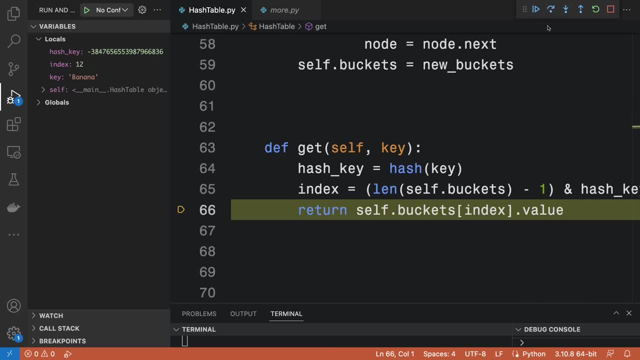 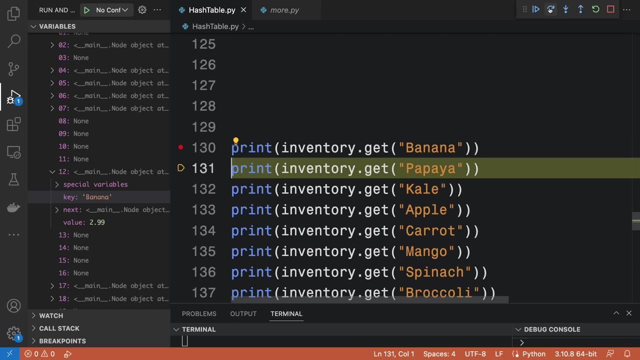 to determine the index where the entry is stored. This tells us that the entry is inside of index number 12.. We can check our bucket's array and it is indeed inside of index number 12.. We return that node's value and then we print it. 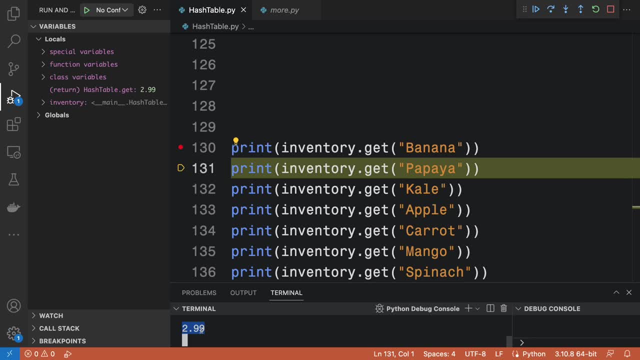 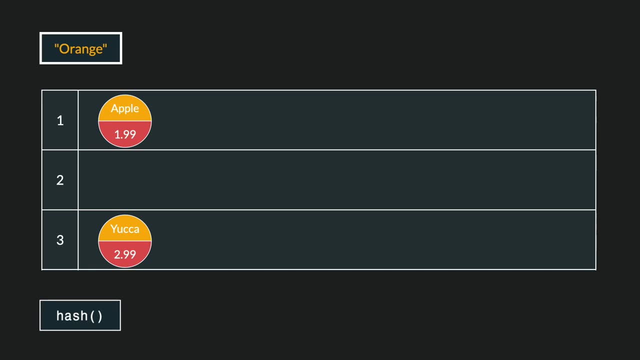 Beautiful. Now, looking at another example, if the user wants to know the price of oranges, once again the key gets processed by the same hash function, The bitwise AND. operation between the hash and the length of the array determine the bucket where it's located. 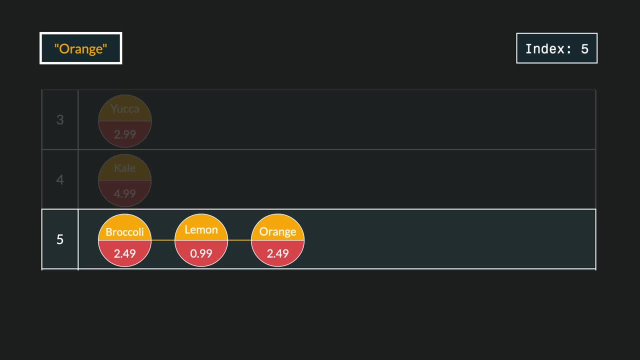 And in the event that a bucket has more than one node, we need to scan through each node, one at a time, until the matching node is located. Once found, the corresponding value can be returned. Now I'd like to retrieve the price of mango. 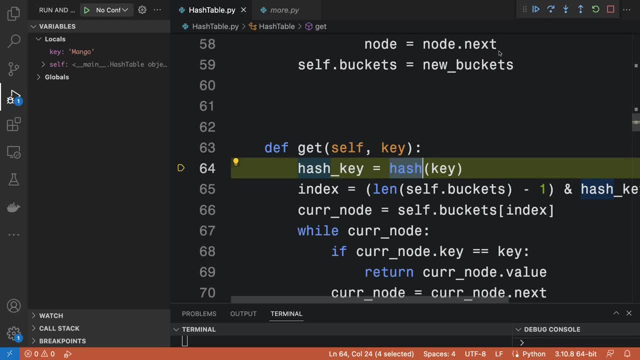 Once again the key gets processed by a hash function to produce the unique hash that corresponds to mango. The bitwise AND operation between the hash and the length of the array is going to determine the index where the entry is stored. The entry for the key, mango, is inside of bucket zero, but if we look inside our bucket's array,